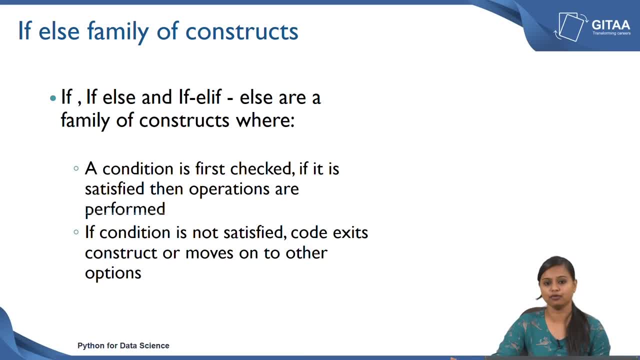 ifs and multiple else clause. the first check would be the condition. Whenever the condition is satisfied, only then the code will be executed or the statement will be executed. otherwise the code exits the construct itself and moves to the other options. So that is how the 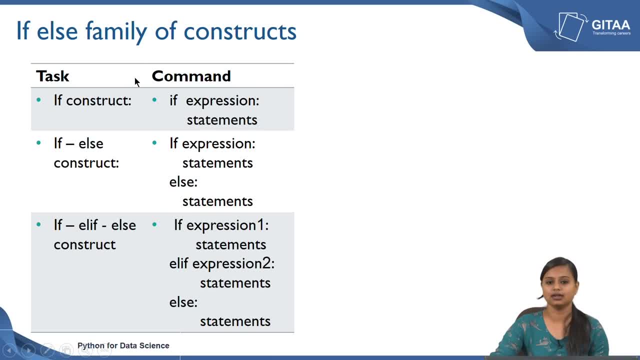 if else family of constructs works. Let us see different task for each construct. So first we look into if construct. the command would be if expression, colon and statements in the next line If as a keyword, if the condition is satisfied, whatever condition you have given. 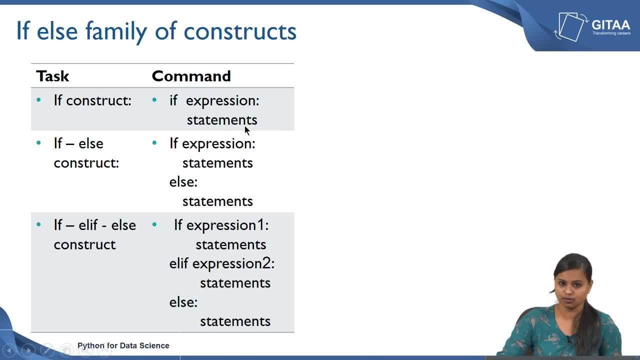 it under the expression, then the statements will get executed. otherwise the code exit the construct itself. Next we will move ahead and see what is the syntax would be for if else construct. It forms the basis from the if construct, wherever we have given the first. 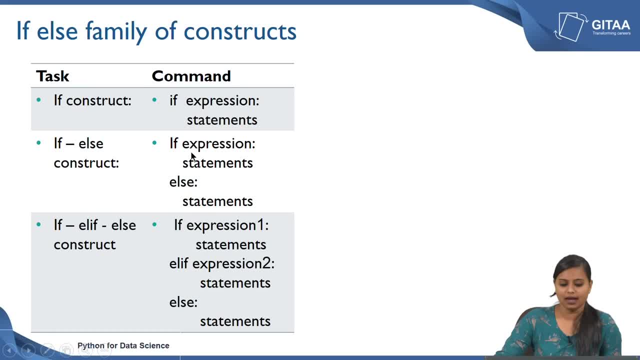 statement using the if keyword and followed by if keyword. you have to give the expression to be checked. that is where the condition to be specified And after that you give the statements that needs to be executed if the condition is satisfied. If the condition is not satisfied, give another statement under the else clause, So using 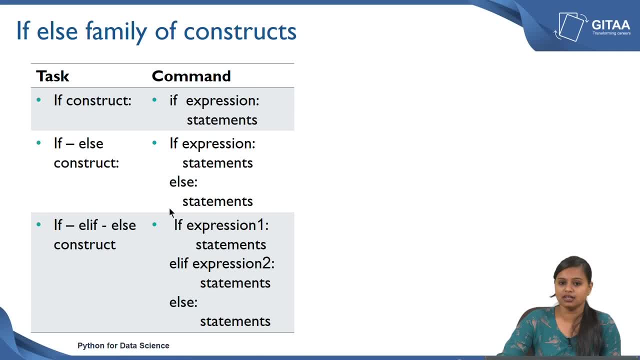 if elif else construct, you can basically give multiple condition that needs to be checked in order to execute a statement or in order to execute any line of code. In that case the command would be like: if expression 1 is being satisfied, then execute the statement. 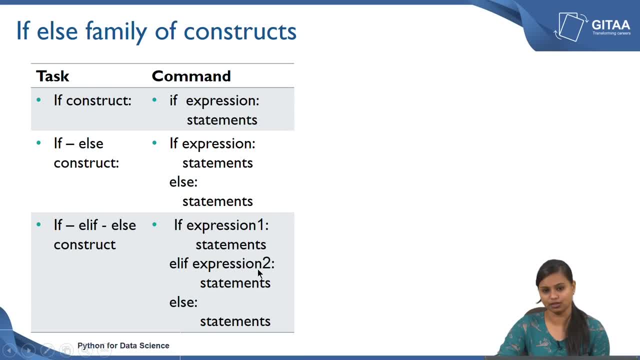 If it is not satisfied, then execute the next condition. if that is not being satisfied, then it also comes to the next else clause where the That statement will get executed. So the else clause statement will get executed only when the other two expressions are not satisfied. basically, the other two conditions are not. 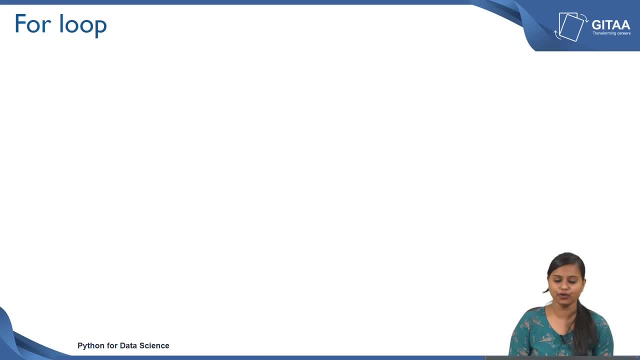 satisfied. So now we will look into for loop. Now we are going to look at the syntax and the different loops here. In the upcoming minutes we will be looking at in terms of an example also. So first we will look at the syntax for for loop. So whenever you 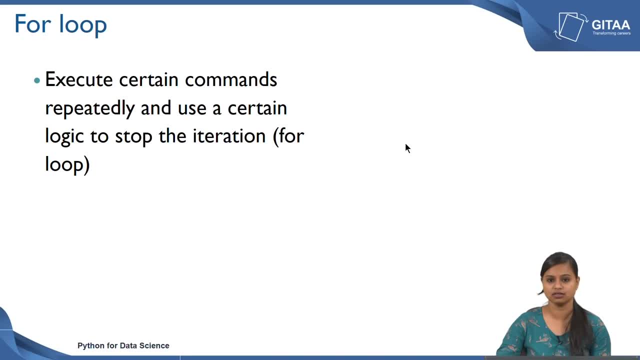 want to execute certain commands Repeatedly and use a certain logic to stop the iteration, you can go for for loop. Let us look at the syntax on how to use the for loop. The command should be like for: iter in sequence colon and followed by statements in the second line. So this is the simple. 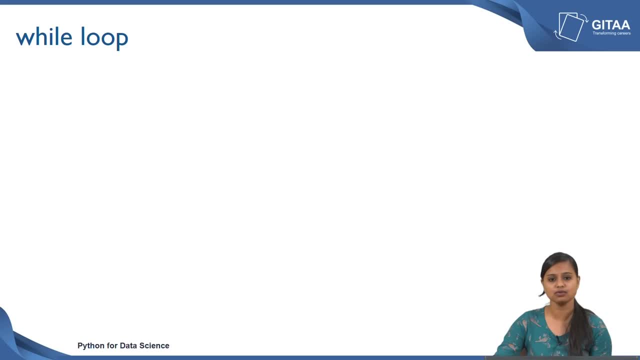 command that is used to construct a for loop. Next, we will see about the while loop and the syntax for while loop. A while loop is used when a set of commands are to be executed depending on a specific condition. Basically, a while loop will be executed as long as a condition is true, Whenever the condition. 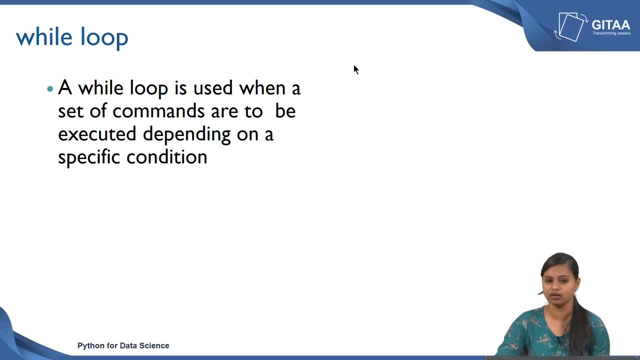 becomes false. whenever the condition you have given becomes false, the while loop execution will stop. So the task being here is the while loop, and the command to construct a while loop is while is the function inside the braces. you have to give the condition And, as long as that condition is true, the statements you have given in terms of statement. 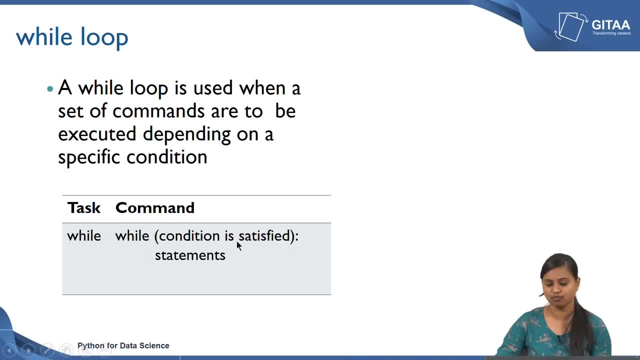 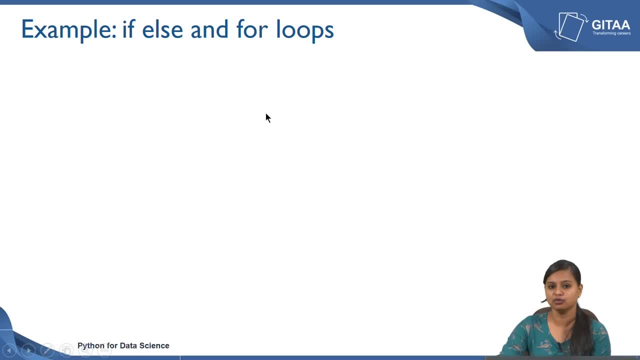 will get executed whenever that condition becomes false. that is when the while loop will get stop executing. So now we are going to see an example to know how we can use if else and for loops. So here we have been working with the data set called Toyota, where we are seeing how 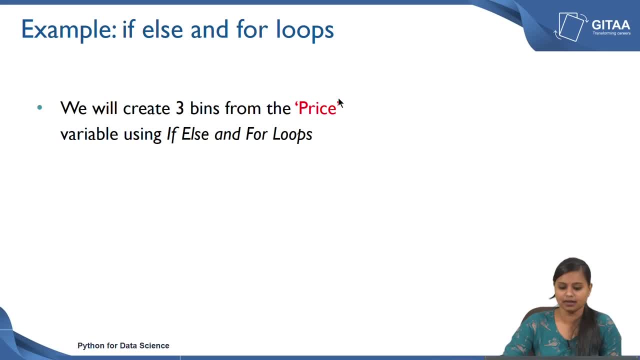 to read them and how to do basic Pandas data frame operations From there. I have just used a single variable called price, which represents the price of the cars, price of the pre owned cars. So I am using the price variable from the Toyota data where I am going to create three. 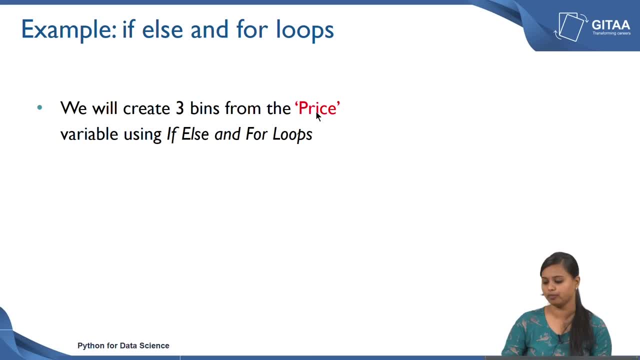 bins from the price variable, using if else and for loops, because the price variable is a continuous variable where it just has the values for the price of the pre owned cars. If I want to segregate those price into three buckets, then I can use if else and for loops. 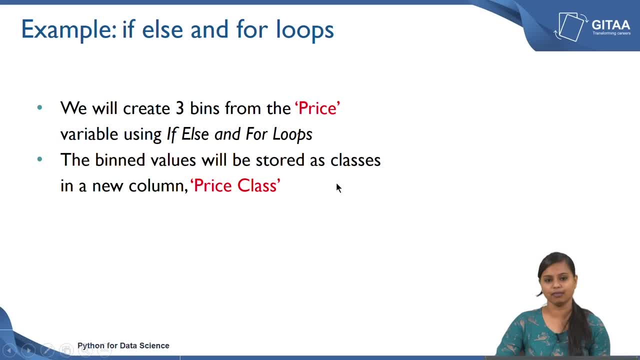 let us see how do we do that: The bin values. as I mentioned, I am going to bin the values, So those bin values will be stored as classes in a new column As price class. so in that case I should be creating a new column to the existing data. 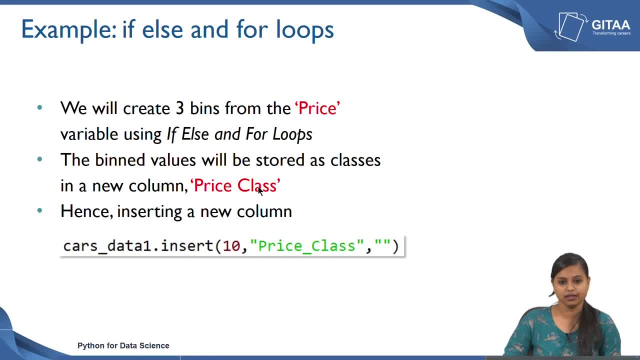 frame. So now I am going to create a new column to the existing Toyota data, where I have read and kept it as cars underscore data 1.. So using the dot insert function, I can give the position to which the column should be. 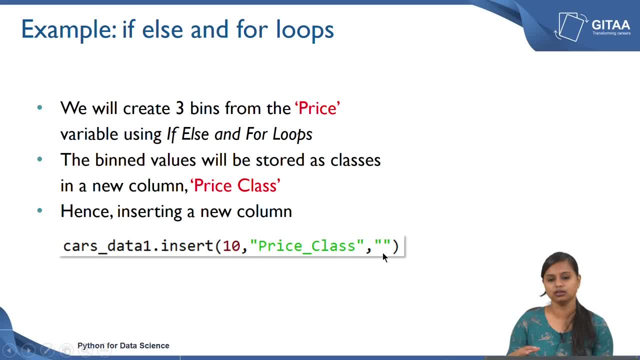 added and the column name and I have given blank, So that all the it will create a column with the blank values. So now a new column has been created as price class so that we can store all the bin values as classes. 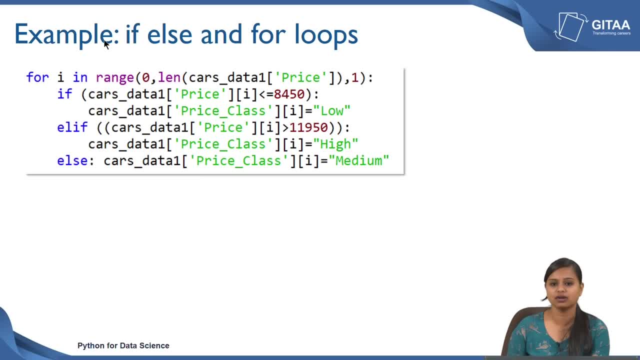 So, using, if else and for loops, I am going to convert all the values into three categories, where the categories represents the range of the price. one is being low and other one is being high and other one is being medium. So if I want to segregate those values into three categories, I want to basically give 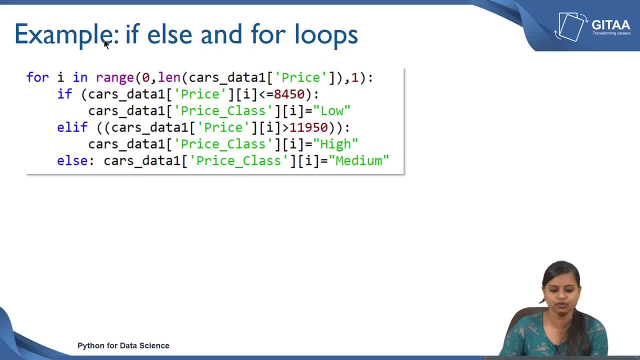 some condition in which it can happen. So I am going to use that. So I am going to use that. So I am going to use that using if statement. So what I am starting here is: I have used the for loop, I have initiated the for loop here, where I have given the iter in sequence: 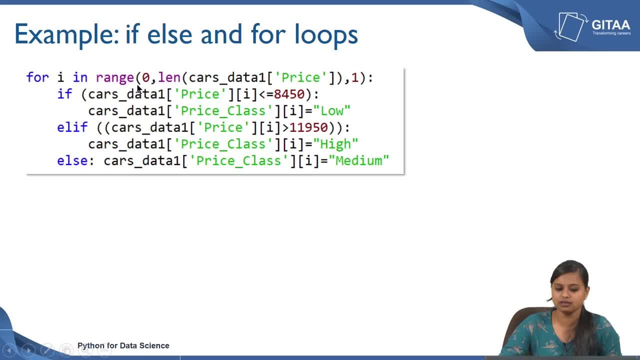 where i is the indexing variable in the sequence. I have given the sequence using the range function, where I have given the starting value as 0 and it should have the value till the length of price. So the value will be 1436 and I have given 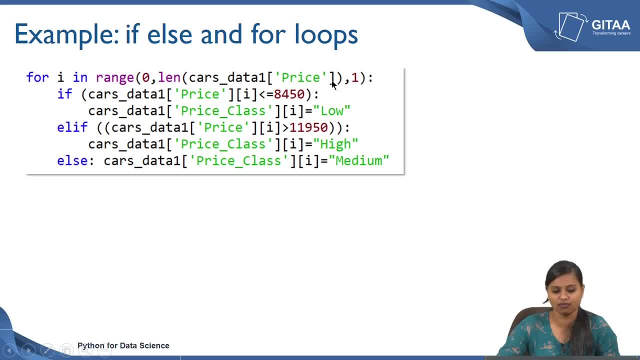 comma 1. then it will. the iteration will happen in steps of 1.. So now I have given from which the iteration should happen, Now I have given the sequence in which the iteration should happen. Now there is a time to give the condition on price, the first condition being I want. 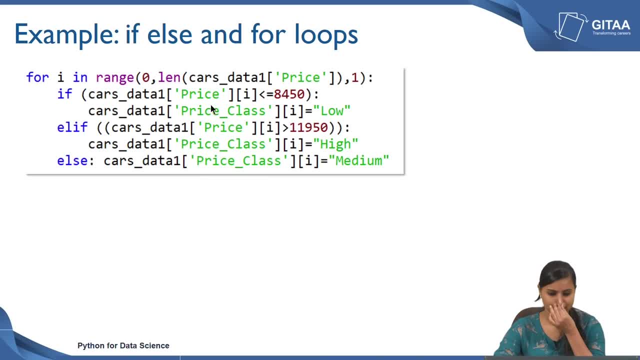 to make. I want to make some records. I want to bucket some records as low by giving the condition: So if the price is less than or equal to 8450, then keep them as in the range low, right? In that case I can just give a condition saying: access the price variable from the cars underscore. 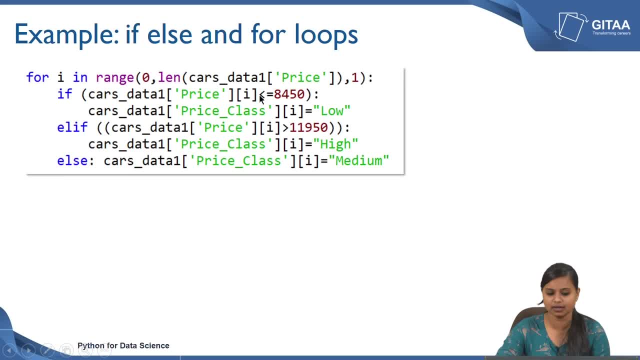 data 1 data frame and give a condition here: whenever it is less than or equal to 8450, then execute this statement. that is, cars underscore data price class becomes low. basically equate a value low To the new variable price class. So this will happen for each and every row and it 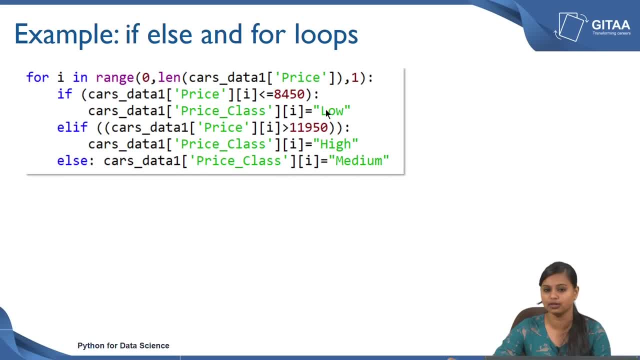 will check whether the price of the cars less than or equal to 8450 or not. if it is, then it basically equate them, equate the value. basically, then it will name the row as low. So there is an another condition, using elif statement, because I need to give two conditions here, one is on low and one is on high. and 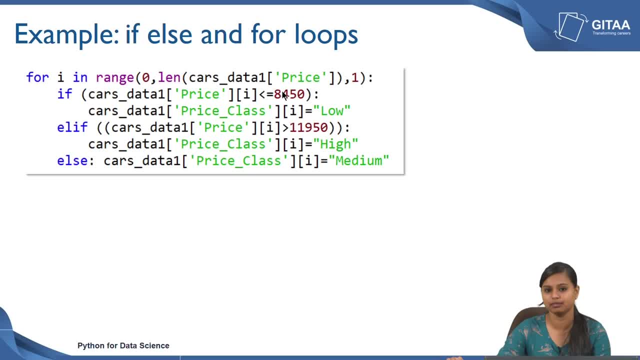 whatever is not being satisfied with low and high, I keep them as medium and all those rows will be kept it as medium. So in this case I have two conditions here. one is price less than or equal to 8450, and the other one is being: whenever the price is greater than 11950, then in that case the 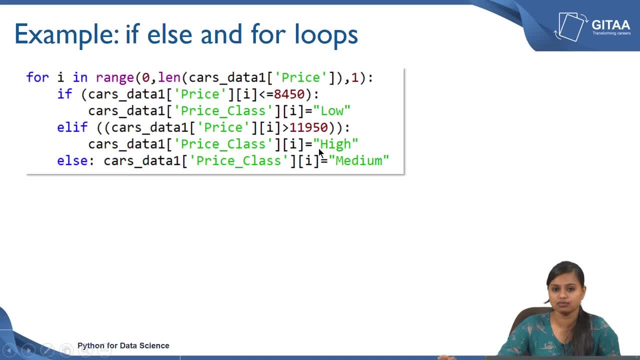 price will be. in that case, those rows will be named as high And that will be stored in the column price underscore class. So whenever these two conditions are not satisfied, whenever any row is greater than 8450 and less than 11950. 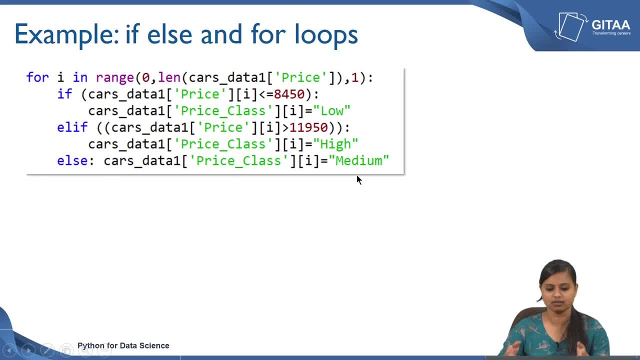 then all those rows will be named as medium. So there is a bound here. So the whatever rows that are being named as medium will have all the rows wherever the price is greater than 8450 and wherever the price is less than or equal to 11950. So this is how I can. 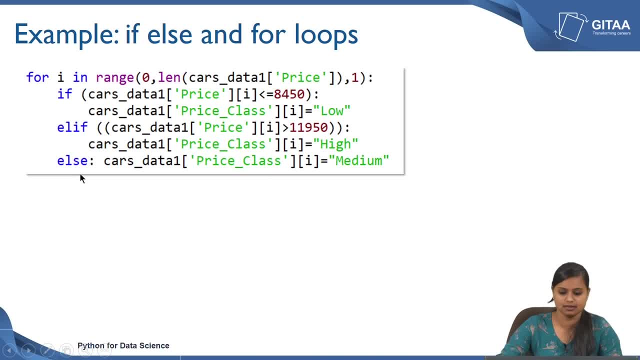 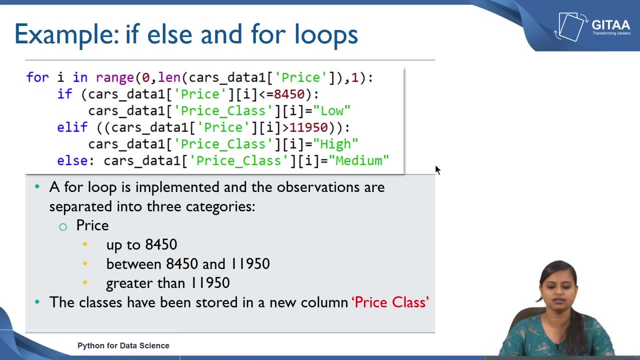 give using for if, elif and else. So if you see that to just to summarize whatever, we have done it in for loop and if else, a for loop is implemented and the observations are separated into three categories right now. So the price being up to 8450 and between 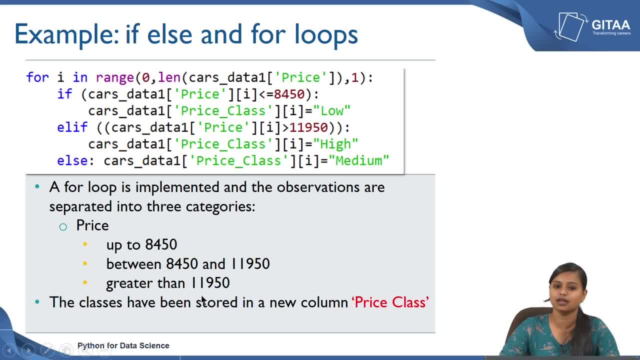 A42 and 8450.. 8450 and 11950 and greater than 11950, and we keep the price less than or equal to 8450 as low and we keep between 8450 and 11950 as medium and whenever the price exceeds 11950. 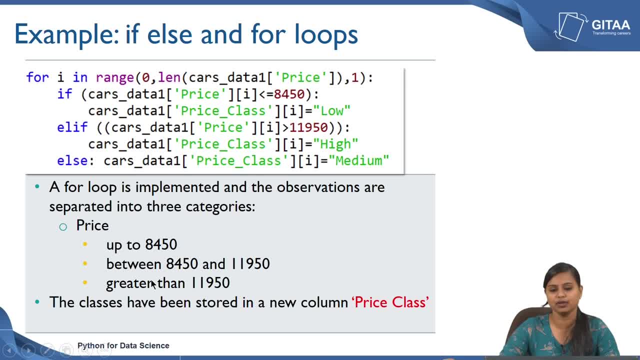 then we keep them as high and we know that the classes have been stored in a new column called price class. So in each of the records of price class there will be a label called low, high or medium that is exactly based on the condition which is being represented. 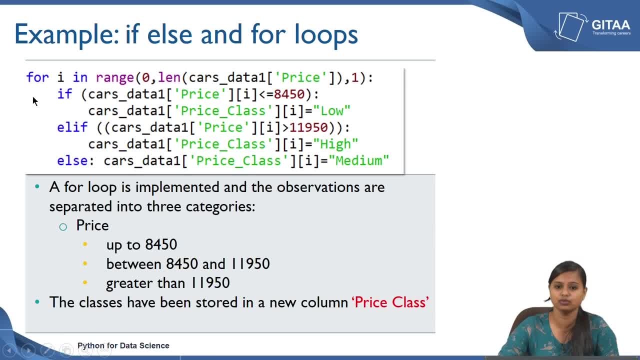 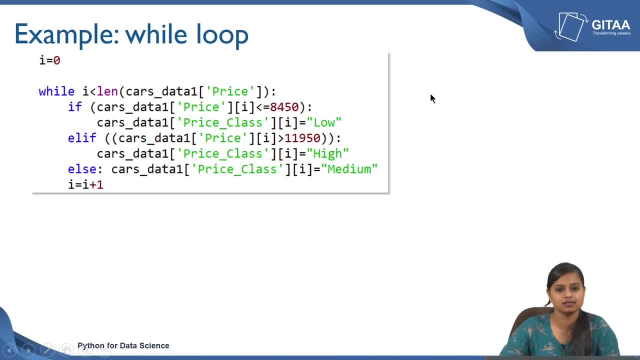 here and we have done that. So, using for loop, we have seen how to do the iteration, and using the if and else clause, we have seen how to give the condition based on a variable. So next, let us see an example for while loop. So a while loop is used whenever you want. 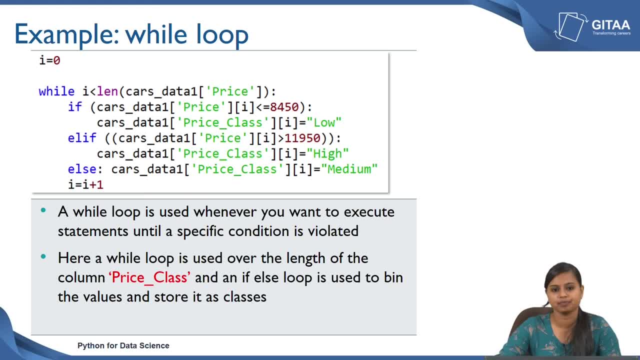 to execute statements until a specific condition is violated. Here I am going to use a while loop over the length of the column, price, class, And, And. if else, loop is used to bin the values and store it as classes. So, whatever we 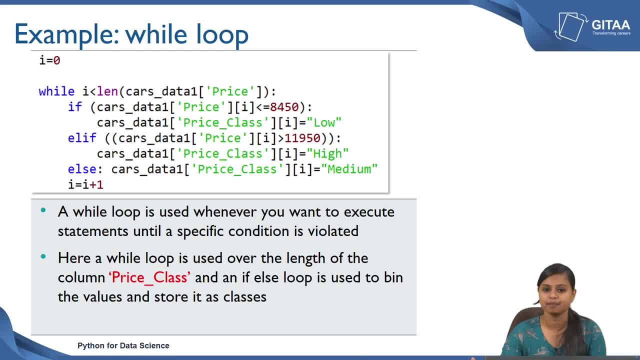 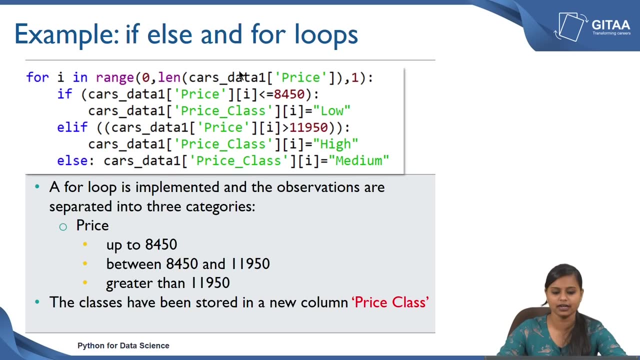 have done it in the previous ah slide. I am going to repeat the same thing using while loop. So you can do that using both for and while. So here I have initialized my indexing variable as 0. the difference between both for and while loop is in the previous slide. 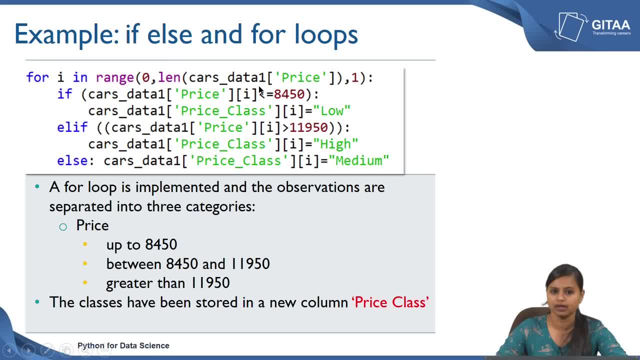 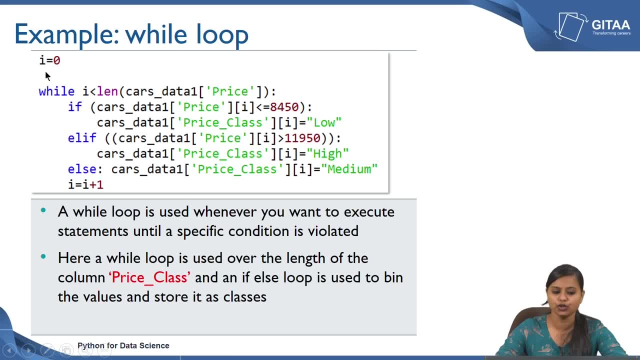 you would have given your iteration step in the sequence itself: Yeah, Using your for, but in this while loop you are giving your, you are just initializing your indexing variable as 0 and you will give the iteration step at the last only because the first check of the while loop is the condition check. 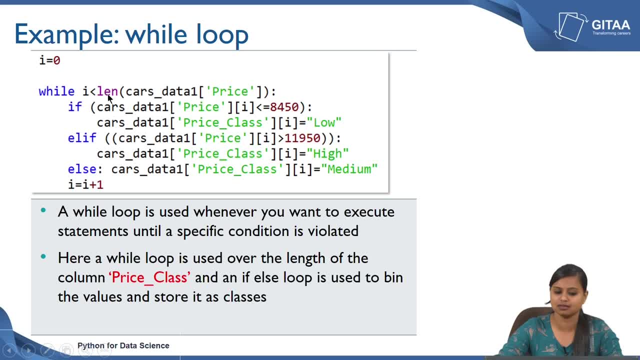 So the while loop will be executed as long as i is less than length of others of data, that is, 1436. The while loop will get stop executing whenever it exceeds the condition. I noticed that I started to give away the the elevation for the x, but I did not take all value of y. 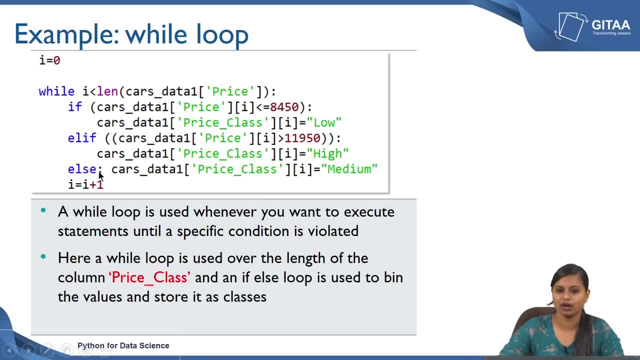 And Yes, Laughing Length of Ming. Let us give 4 vengeance features ____". Let us say while loop that condition: Whenever your i becomes 1, 4, 3, 7, your while loop will get stop executing. 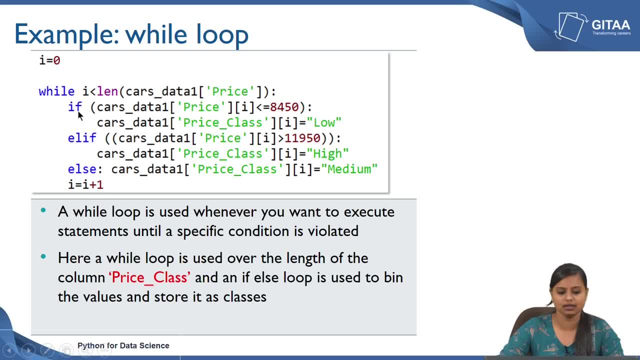 So next, I have a condition here, the same condition being represented here, with the same if elif and else clause. The difference being here is you give the iteration steps at the end of the loop whenever you you are using a while loop and you give the iteration. 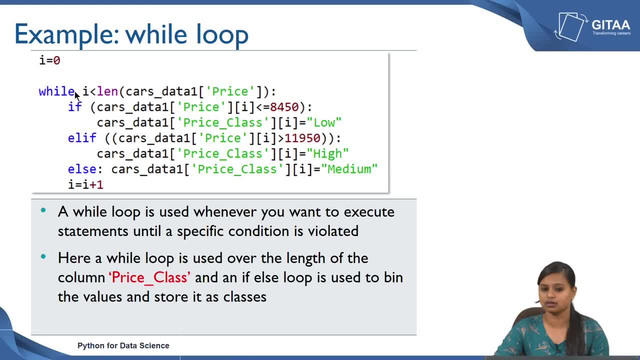 steps at the beginning of the loop itself, using a for loop. So here, if you recall, whenever the price is less than or equal to 8, 4, 5, 0, then keep them as low under the column price class, and whenever it it is it exceeds 11950, then keep them as high under the variable. 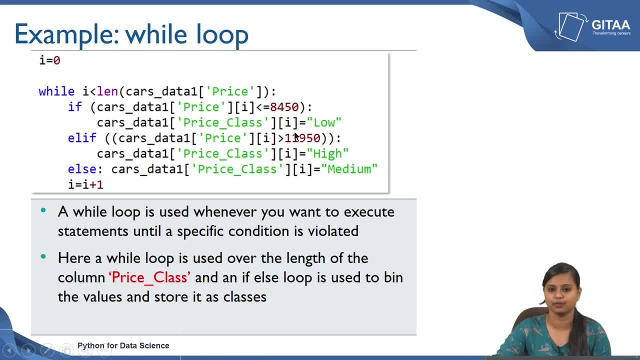 price clause and whenever both the conditions are not satisfied, whenever the price is greater than 8, 4, 5, 0 and less than or equal to 1, 1, 9, 5, 0. Then in that case that observations will be named as medium. So now we have seen the 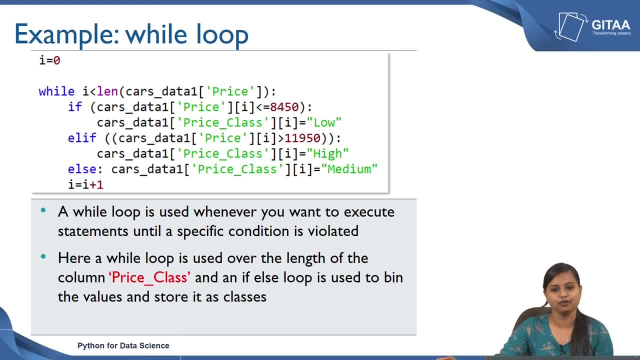 examples for both for loop and while loop to basically bucket all the price values into three categories as low, high and medium. There might be other functions which will do it thereby. there are so many inbuilt function that does this. but using a for loop, when 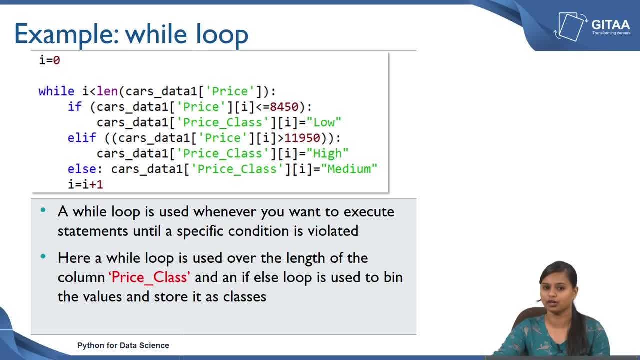 you have a control on whatever you are doing with the steps. then you can use the for loop and while loop. We have now three bins, now three categories now: low, high and medium. So we do not know how many records fall into row and how many records fall into low and how many records. 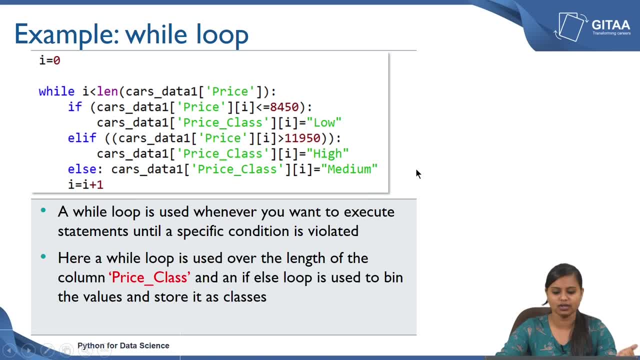 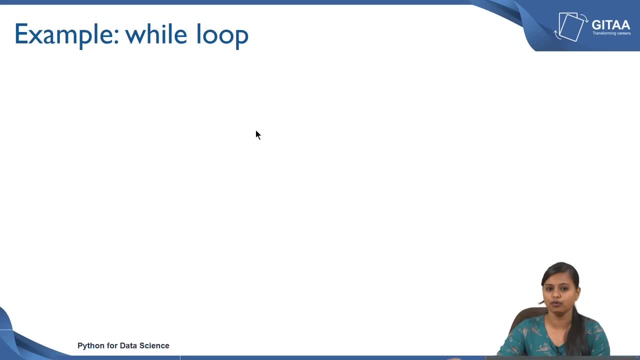 fall into high and how many of them fall into medium. So let us just see how your observations have been categorized. So now we basically used a loop to combine all the price values into three categories: one as low, medium and high. Now I want to check how the categories 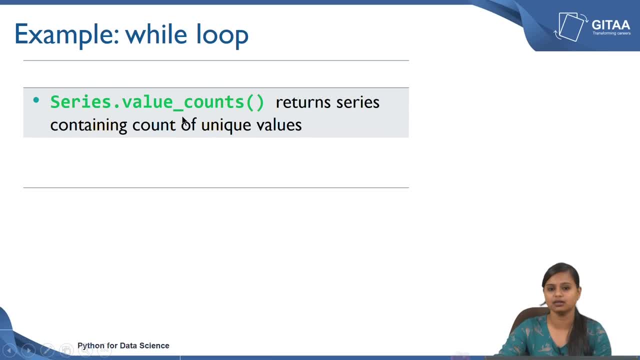 have been categorized, So in that case I will be looking at frequencies of each categories. that is, low, medium and high. I can get the frequencies of each categories using value underscore counts function, So whenever you have a series you can use value underscore. 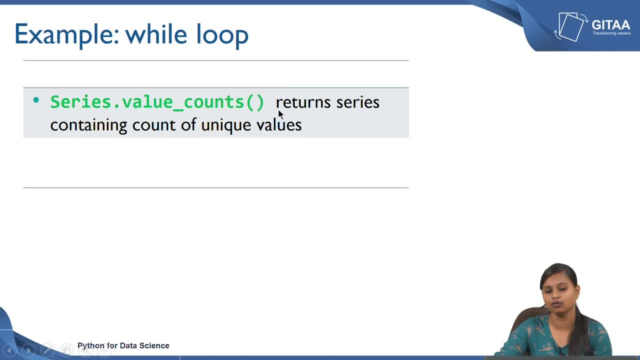 counts that basically return series containing the count of unique values. I want to check the count of unique values under the price class, that is the variable name and cars underscore data. one is the change, So I can see the change in value. and then I want to check the. 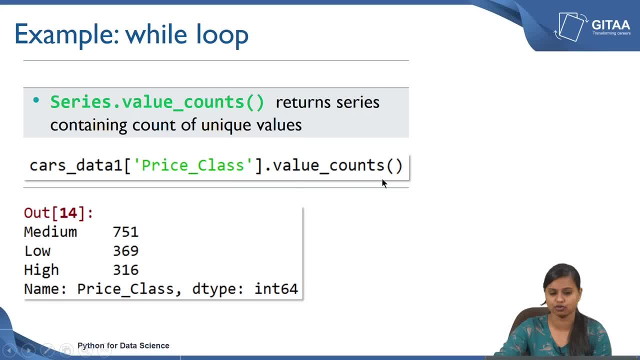 data frame name and dot value underscore counts as the function. if you use that, it basically gives an output which is shown here. So you have 751 observation that falls under the medium category. that is basically those cars are in the range of medium, those cars have the price in the range of medium and 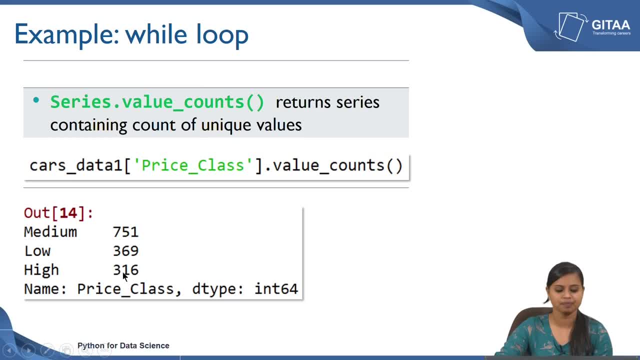 you have 369 observation with the low range and you have only 316 observation with the high range, and the name being price class and the data type of the output is being in 64. So now we have seen how to basically convert your numerical values into a categorical variable. 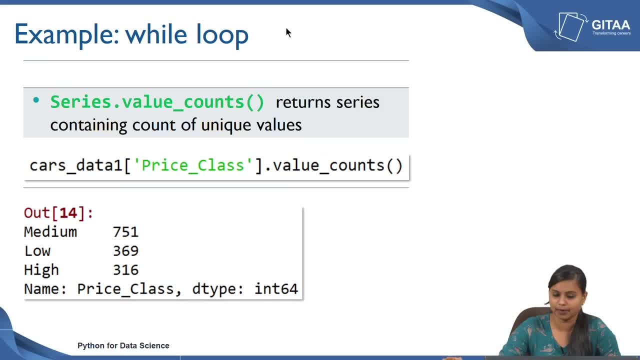 right, because now we have converted the numerical variable price into categories as low, medium and high. that becomes a categorical variable. now that is why we have checked the unique count of each categories. So you can. if you want to do that, you can use either a for loop or a while loop. 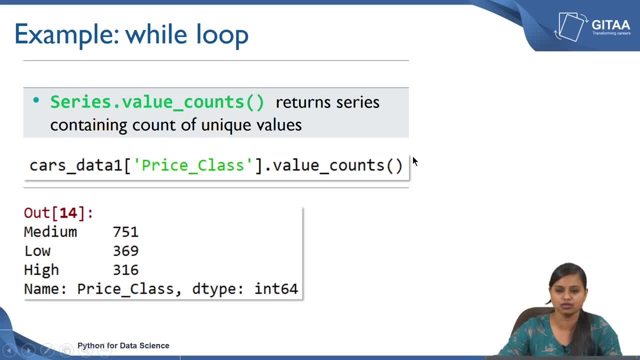 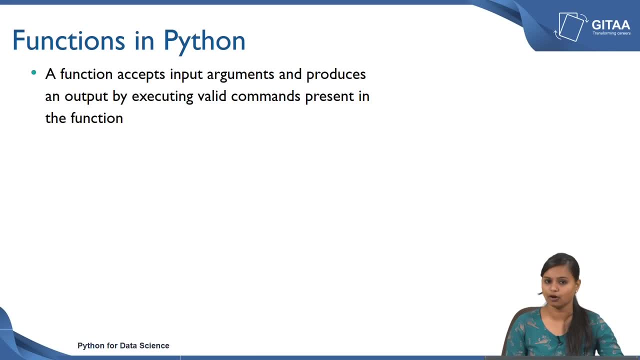 So this is where all the while loop and for loop comes into play. Let us see about the functions in python. basically, a function accepts input arguments and produces an output by executing the valid commands present in that function. and the function name and the file name need not be of the same, because you can have a different file. 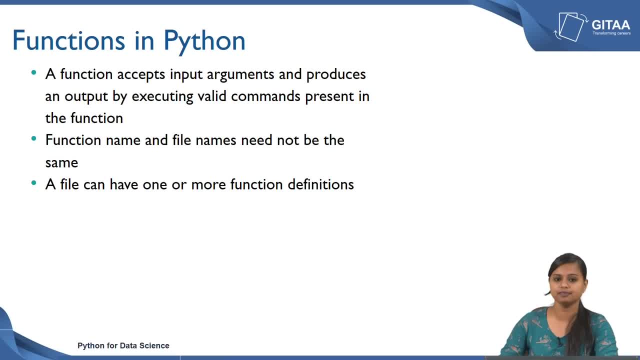 name and a different function name. that holds good in python and a file name can have one or more function definition. So if you have a file where you defined a function, That function file can have one or more function definition. there would not be any issues. 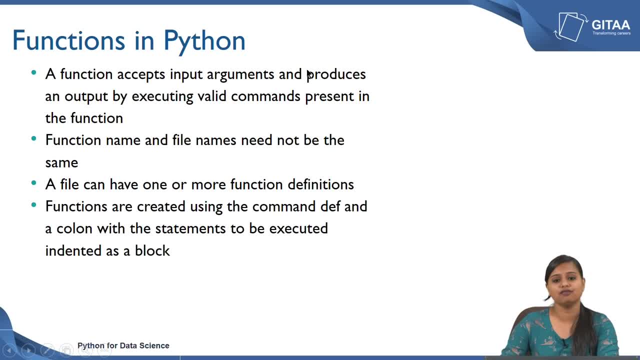 while you are calling a function in a different file and the functions are created using the command def and a colon with the statements to be executed in intended as a block. So this is how you define a function: you use a def function and the function name is: 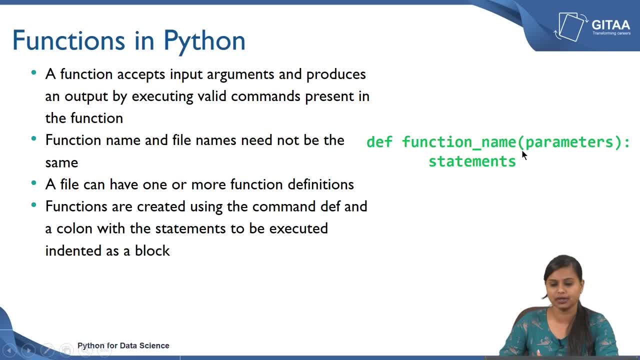 followed by that. So, inside the parenthesis, you basically need to give the parameters based on which your calculations will be done. So, using the statements here, you will give the basically an equation or an expression that should be calculated, that should be solved, based on the parameters that you have given. 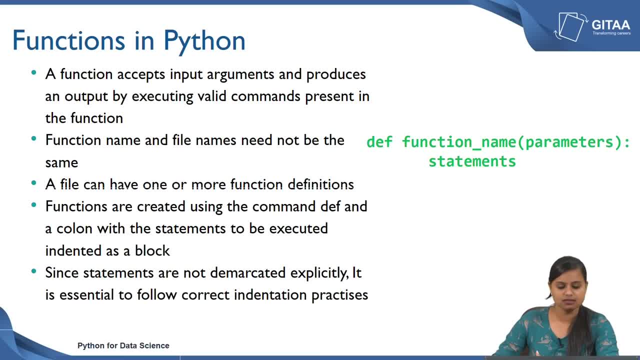 inside the function name parameters And since the statements are not demarcated explicitly, it is essential to follow correct indentation practices because other programming languages, the python, does not support the curly braces for any control structures or function, So it uses the indentation to explicitly show the demarcation. so the indentation should. 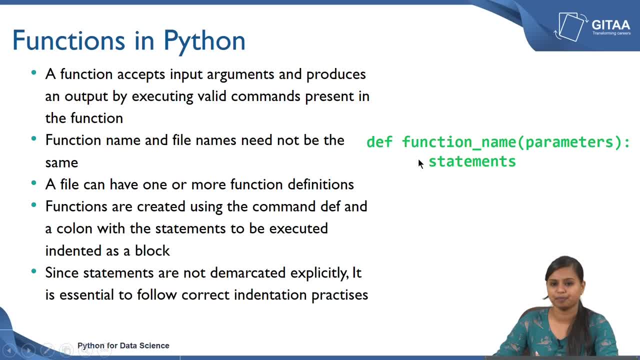 be followed. So your statement should be exactly slightly away from your first three letters of your function name. whenever you type a colon and give an enter, it will automatically comes with an indentation, So it is suggested to not to change that indentation. So now let us see an example on how to define a function. 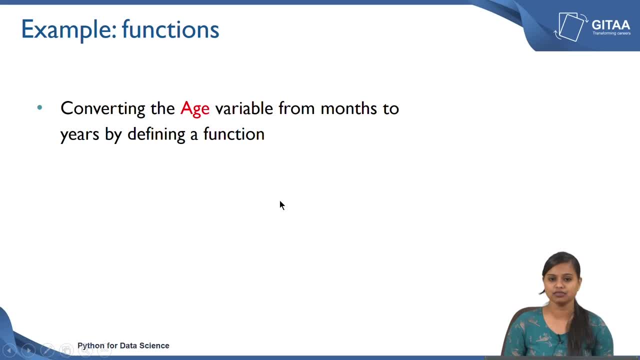 So I am going to define a function which will allow us to convert the age variable from months to years. by defining a function, I am also using the age variable from the Toyota Toyota data that we have, that we are working with. So in that case, age is being represented in terms of months, but that does not convey. 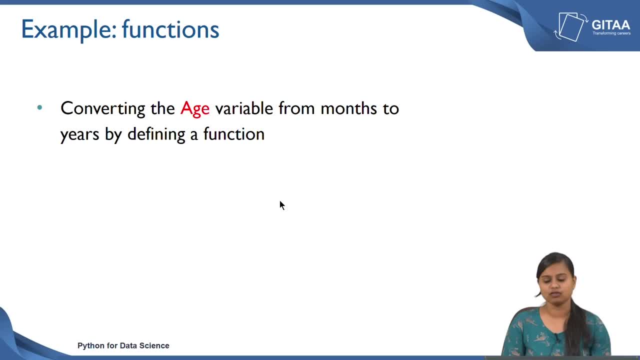 me the exact information or the efficient information, but that is not the exact way where I can infer the age in. rather than keeping the age in terms of months, I can also keep the age in years, So I want to convert the age variable from months to years by defining a function. 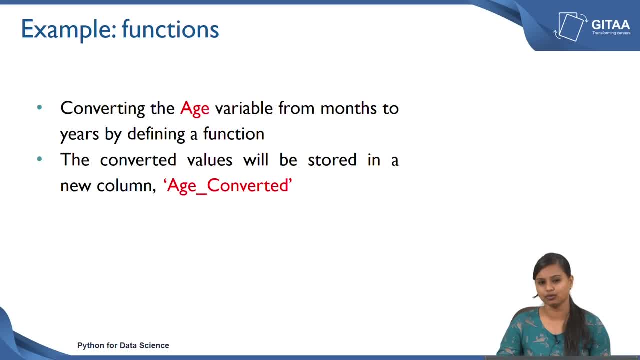 So the converted values should be stored in a new column. So I do not want to attach the existing column. rather, I am going to store all the values in a new column called age converted. So I should be creating a new column called age converted now. 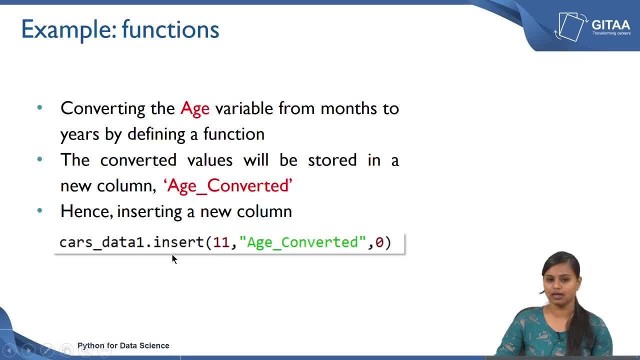 So I have created age converted using the same dot insert function where I want to keep the age converted and 11th position, And initially I want to have all the variables values as 0. that is what I have given as 0 here. 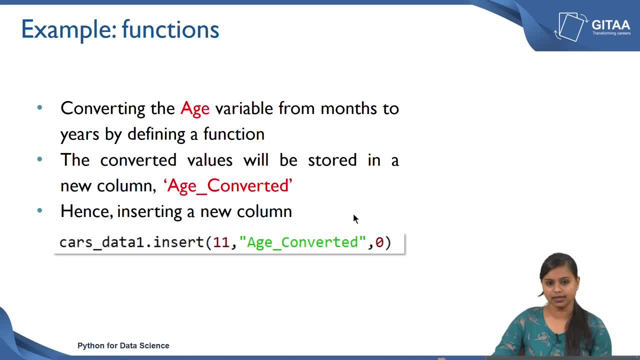 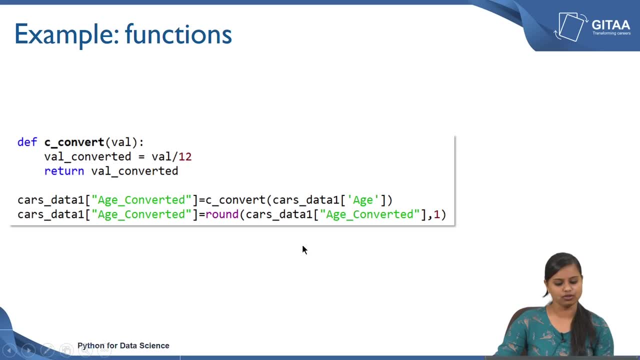 So once you have executed this line, a new column will be created as age converted. So now let us define a function to convert the age from months to years. So here I am defining a function, c underscore convert, and the function takes arguments and: 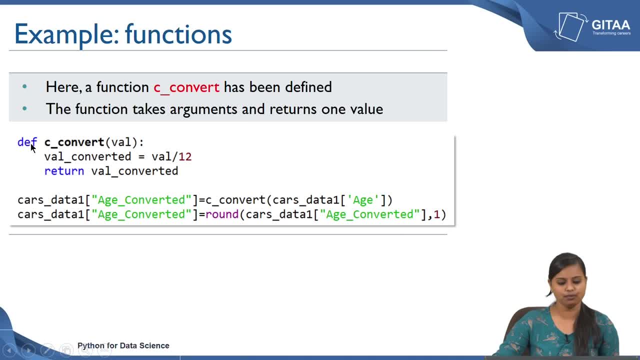 returns only one value. So def is the keyword that is used to create a function definition or the command that is used to function that is used to create a function definition and the function name is c, underscore convert and inside the function I have given the argument called val v a l. 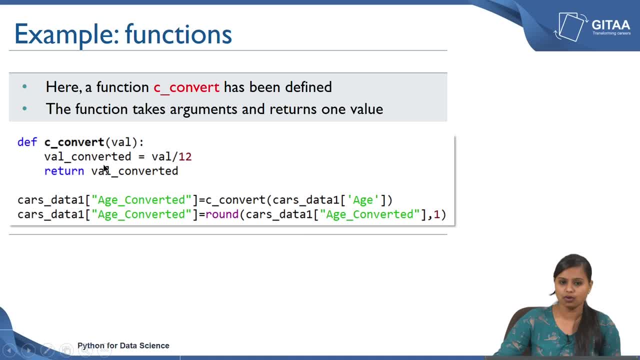 and followed by a semicolon in the next line. I have a variable called v a l, underscore converted. that represents value converted. How am I going to convert? I am going to convert that value by dividing whatever value that is given here by 12.. 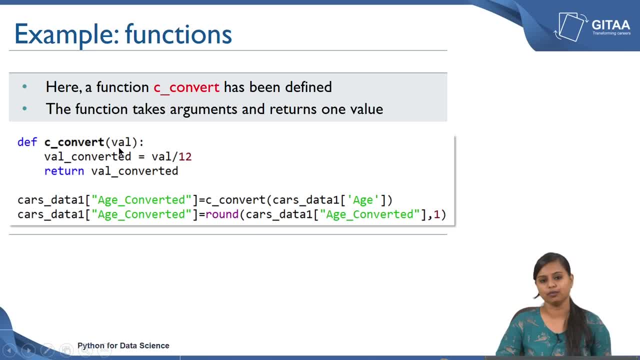 So this is the value. This is the default argument. So whenever you call any function, you can use a c- convert and give a variable there or give a value there. that will be divided by 12 and it will return the value- converted value- and it will return the value or that is stored in the val underscore converted. 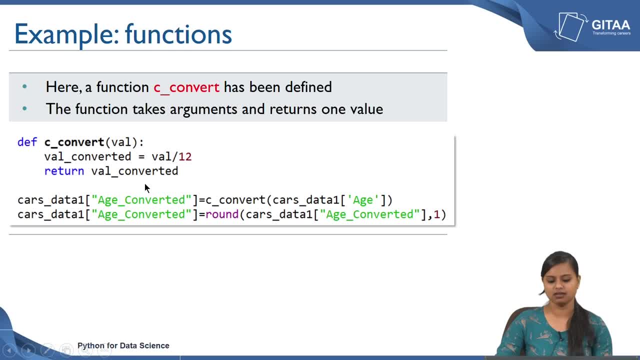 So now, using this function definition, I can basically convert the age variable into months. I can basically convert the age variable from months to years. How I can basically use the same function here, that is, c, underscore, convert, and inside the function I just basically need to pass in the arguments for val to divide any number. 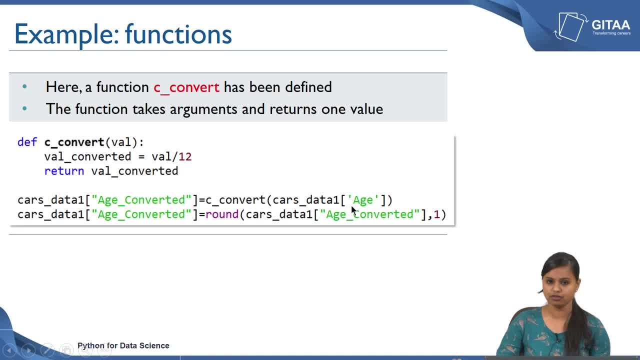 by 12.. So I want to divide all the numbers from age by 12.. So I have given cars underscore data 1 of age. So all the observations under the age column will be divided by 12. So that I get the age converted to years. 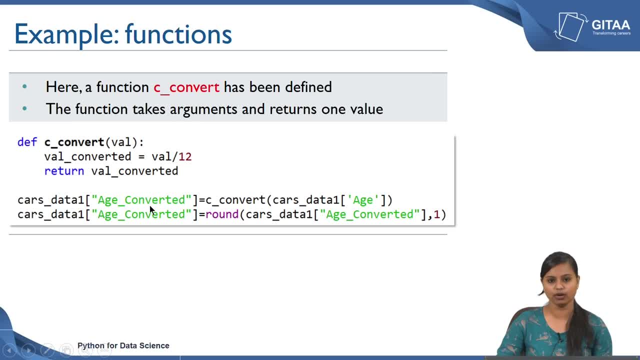 So, if you see, I am storing that into this. I am storing that into the new column called age underscore converter from the data frame cars underscore data. So this will, this new variable will have all the age has been converted into years. and whenever you are doing any numerical operation, python always comes with 5 to 6 decimal points. 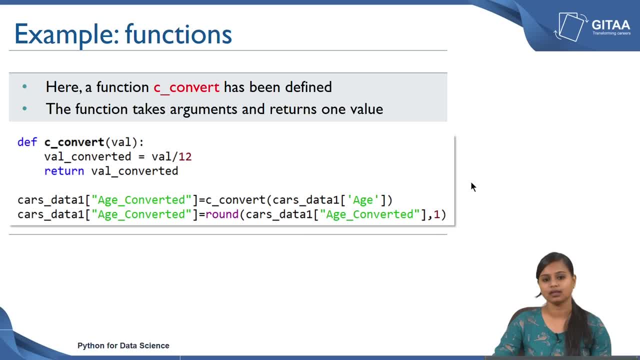 I do not want to have a variable which has so many decimal. that also does not convey the exact information of year. So I want to round it off to only one decimal, So that So it does not have 5 to 6 decimal point, it will just have a digit after a decimal. 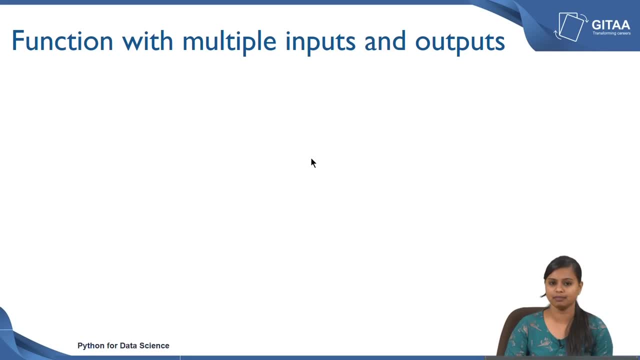 point. So till now we have been seeing about a function which accept a single argument or multiple arguments and which will arrive at a output value- single output value. Now we are going to move ahead and see how to define a function with multiple inputs and arrive at a multiple outputs. So function in python takes multiple input objects, but 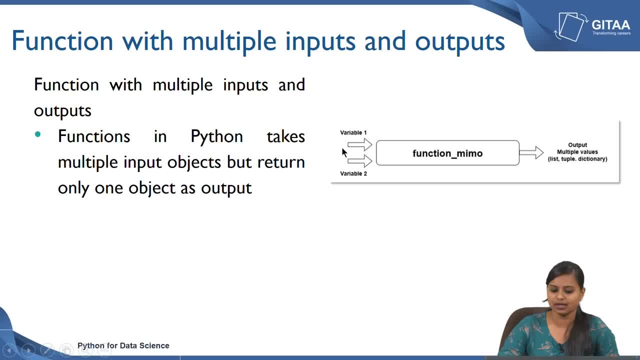 return only one object as output. So you can have variable 1 and variable 2 as inputs to your function, but your output will be in a form of only single object. but that object can contain multiple values, like a list can contain multiple elements and a tuple. 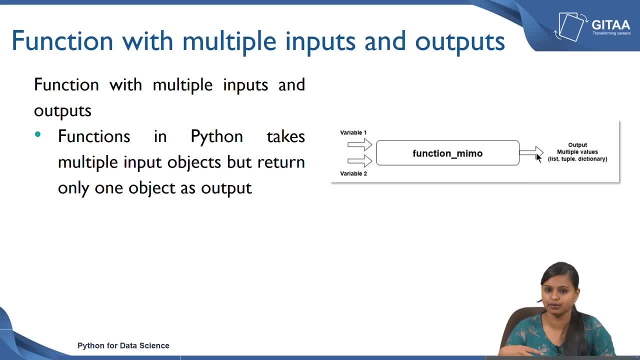 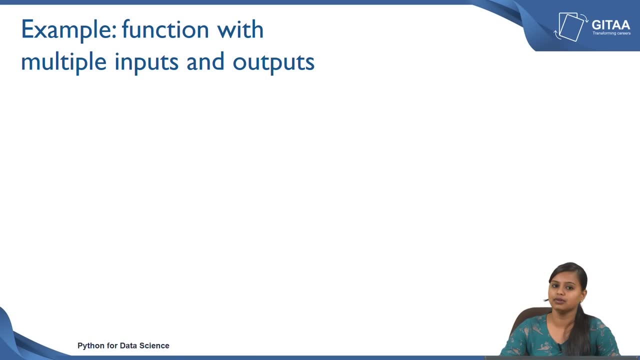 can contain multiple elements and a dictionary can have multiple keys and values, So in that case you will have multiple results in form of a single object. So, like I said, list tuples or dictionaries can be used to return multiple output as required. Let us see an example to see how function with multiple inputs and output works. 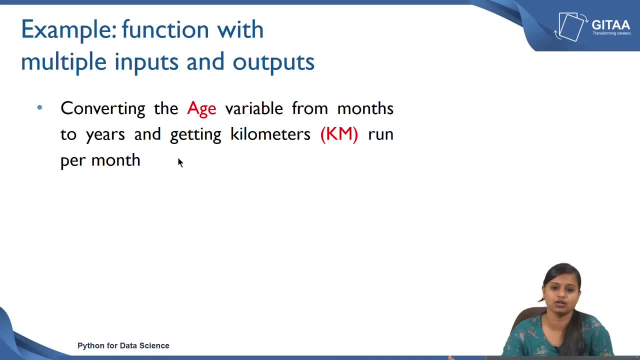 So here, by defining function with multiple inputs and outputs, I am going to do two things: one is converting age variable from months to years, and another one is getting kilometers run per month. So the values of kilometer will be stored in a new column called km underscore per month. 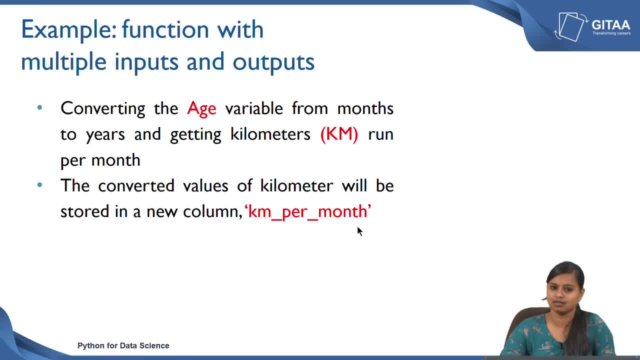 We have already created one new variable for age as age converted, So I am just going to create one more for kilometer per month. That is also using the same insert function, where I have set the position for the kilometer per month variable and the variable name being: 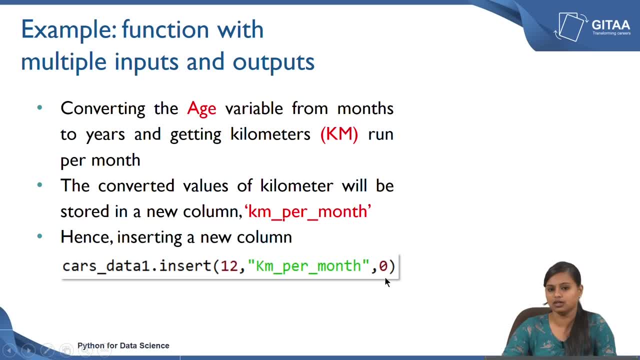 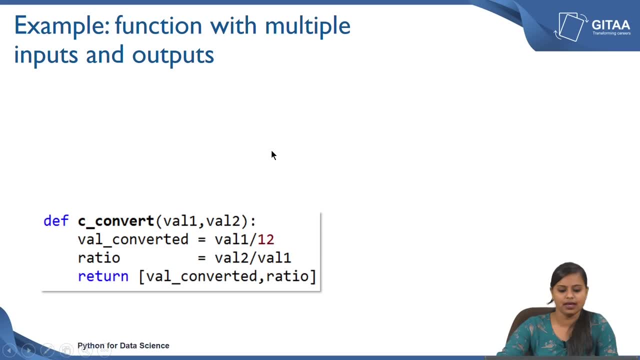 kilometer per month, and I need to fill basically all the values with zeros initially. So I have given 0 here. So now let us define a function which accepts multiple arguments and which will also give us multiple results as a single object. 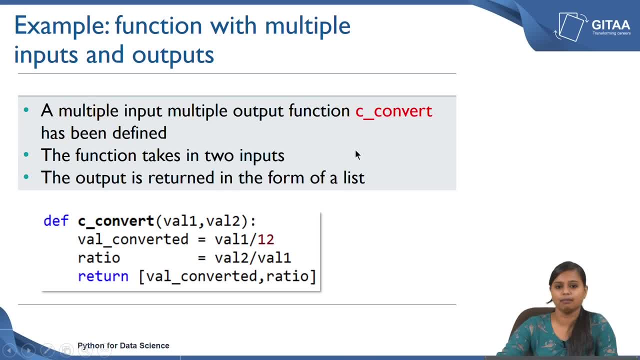 So here is the function definition. So, as I mentioned, a multiple input, multiple output function c underscore convert has been defined. This is the function c underscore convert, and the function also takes in two inputs, value 1 and value 2, and the output. 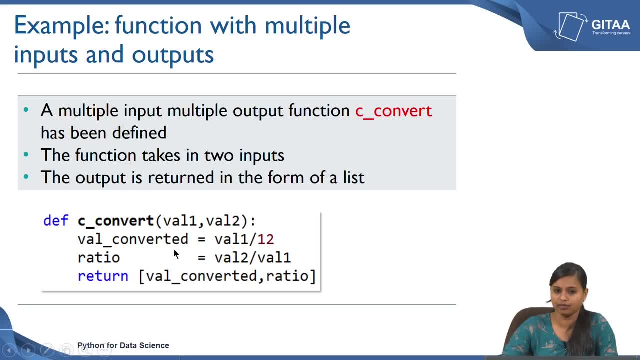 is going to be returned in the form of a list. that is how I have defined the function. If you see, from the start I have defined a function called c underscore convert. I have given two inputs here- value 1, value 2- and I am going to get two output. 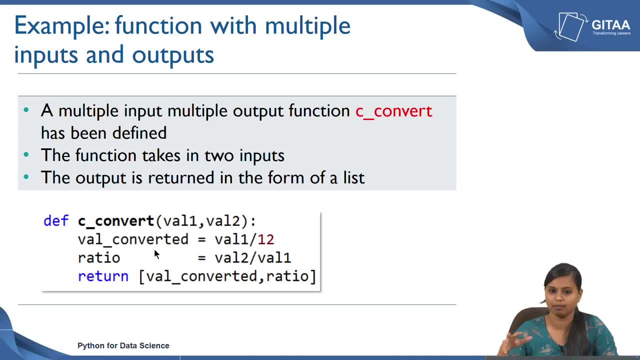 One is value converted from for the age from months to years, and the other one is the ratio. So val 1 and val 1 divided by 12 basically divides all the observations under the age variable and give you an output that would be stored in pal underscore converter. So 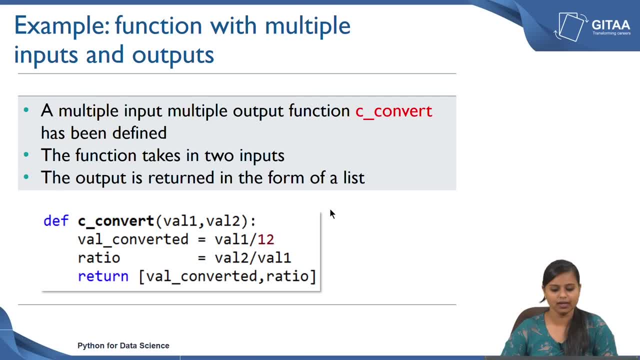 And now I have created another variable called ratio, where my interest is to convert all the kilometers run per month. So in that case I am going to divide each and every observations of the kilometer by the value 1, where I am going to divide value 2 by value 1.. 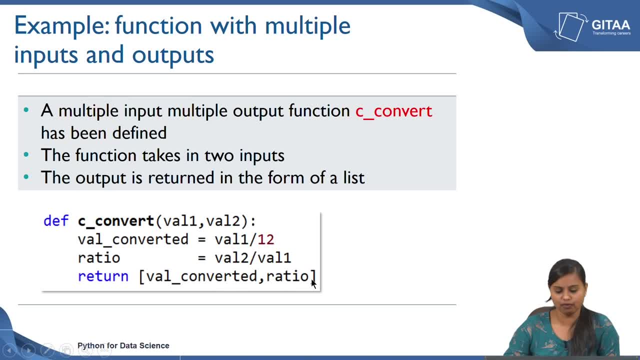 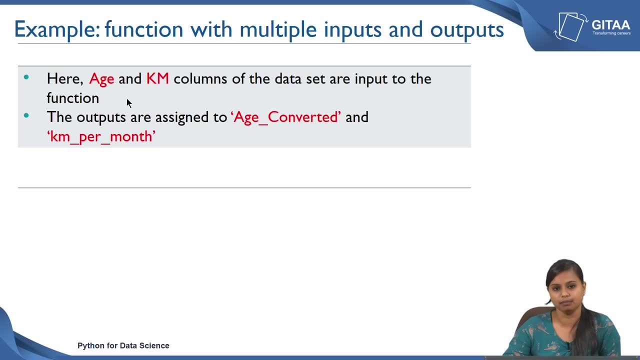 And it will return both value converter and ratio in a form of list, because I have given the values inside the square brackets so that the value will be returned in a form of list. So let us see how do we do that. So here, age and kilometer columns of the data set are going to be the input to the 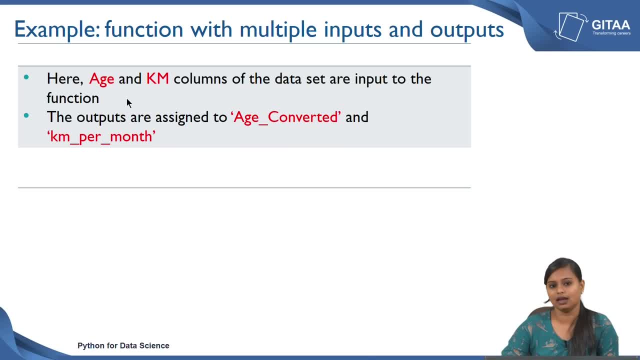 function because I am going to convert age from months to years, I am going to convert kilometers run and I am going to get the kilometers run per month And the outputs are going to be assigned to age converted and kilometer per month, where 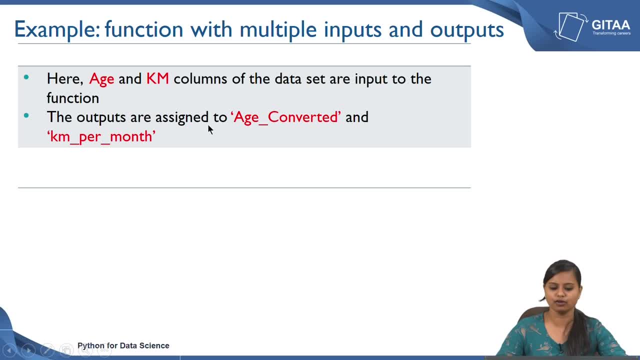 we have created two new variables, And here the outputs are going to be assigned to age converted And kilometer per month, because I am going to save my output simultaneously. So, as you know, in python you can assign multiple values to by giving multiple variable links. 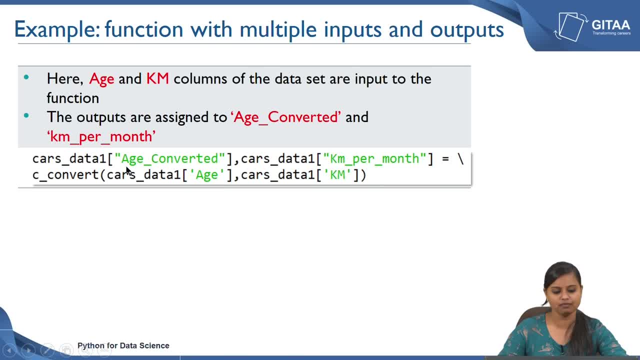 So that is what I am going to given here. So here the variable. the first variable name is age, converted from the data frame cars underscore data 1.. And the second variable is kilometer per month from the cars underscore data 1.. 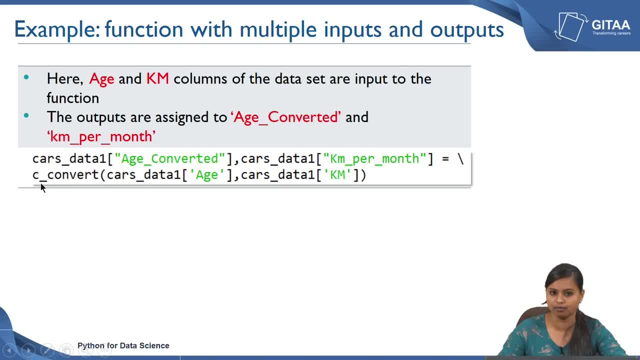 And what I am going to save here is the output from the c underscore convert function, which I have defined it in the previous slide. So c underscore convert is the function and the input would be cars underscore data of age. So age will be the first input and the kilometer would be the second input. 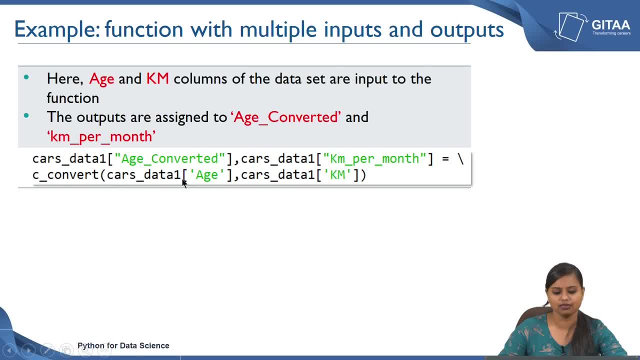 And I have stored whatever value. I am getting it using the first argument as age converted to age converted, and whatever I will get it using the secondvariable will be stored in to the second variable called kilometer per month. So let us look at an output after using the c convert function. 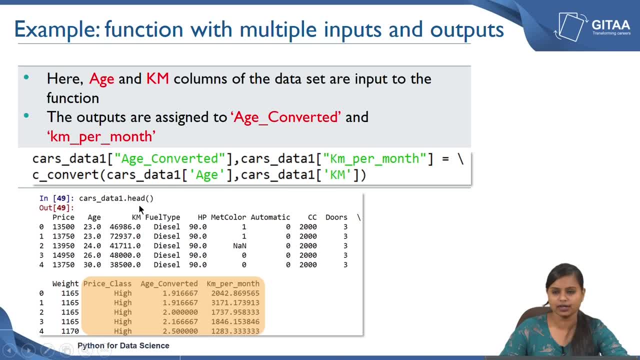 What is the output that we are likely to get? I have used dot head function to basically look the first five rows of my data frame just to see how my variables have been populated. So if you see the price class, this is using the for loop and while loop which we have. 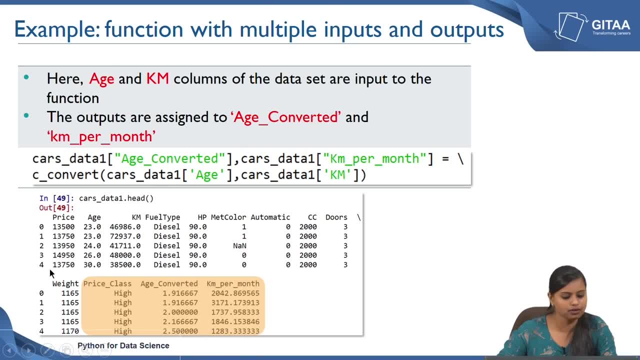 given here. we have a bucketed all the price values. If you look at here, there are price values like 13,500.. We have given some conditions where if it exceeds some value, then keep it as high, low and medium. Then in that case the first five rows have been stored as high and if you see we have 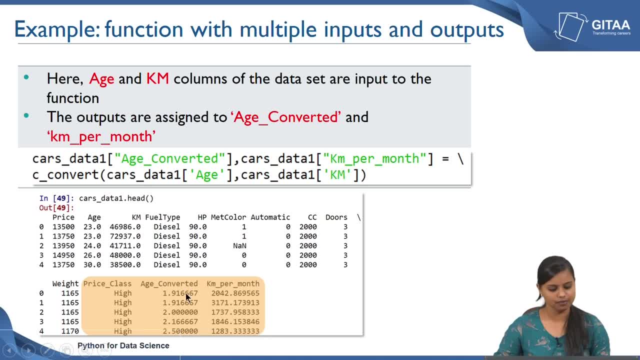 converted the age, which were in months, to years. I have just divided every row with twelve, So I got 1.916667.. see here, this is not the rounded off value. So this snippet just gives you the output with 5 decimal values. you can also round that to 1 decimal point, because this value does.